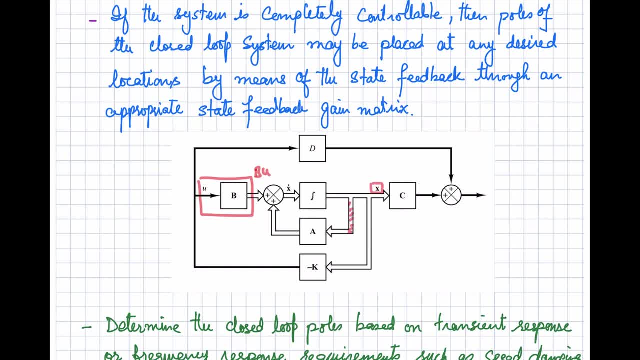 this point we have the X. so through this feedback path we have A into X right and at this position we have X dot. so what is this X dot? X dot is equal to AX plus BU right. so BU is over here, this one, and AX is coming from here. so here we. 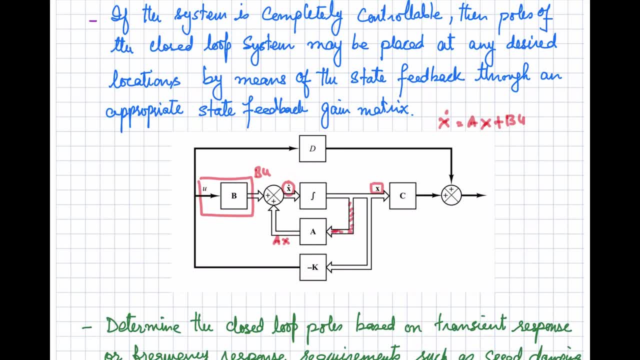 have the summer. these two are added up to get X dot and if we integrate this one X dot so we will get the X. so this loop, this portion is basically, is implementing that aX plus BU there is equal to X dot and then from this X dot by integration, you are going to get X. 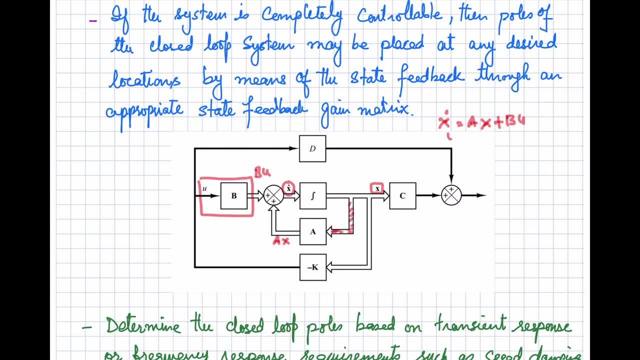 and the output equation in your state space is equal to CX plus DU. so here you can see, at this point what we have. the input is X, X, punto. here we are going to get B, U, we automatically Qin yin. so output will be c into x, right, and this is being fed to the summer and over. here we have 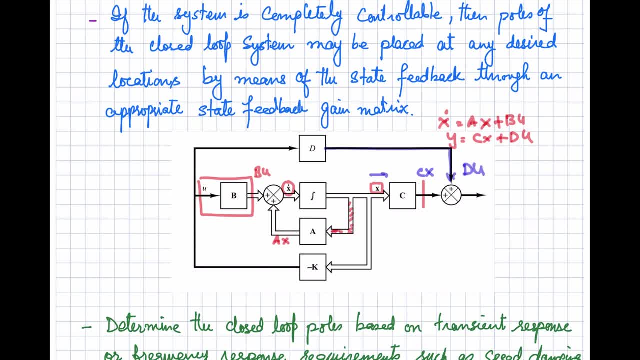 the input d into u, because over here we have the u, so this block will multiply this u with d and that will be available over here. and so finally, over here we have the y, that is, c, x plus d, u. now, if all the states of the system are available for the feedback, right, so over here. 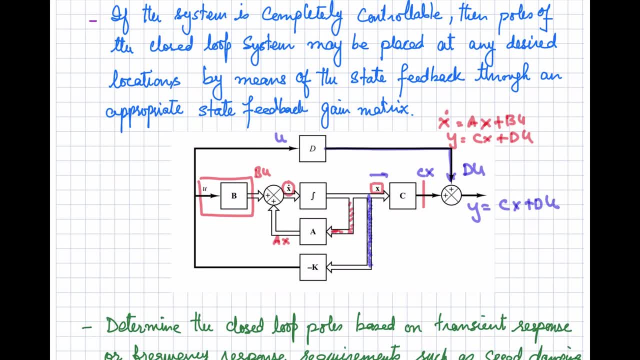 you can see, the x, x is these set of your state variables. if all the state variables are available for the feedback, then we can design this controller having the gain k, which will define an input such that we can set our closed loop poles at the desired position, because it is a completely 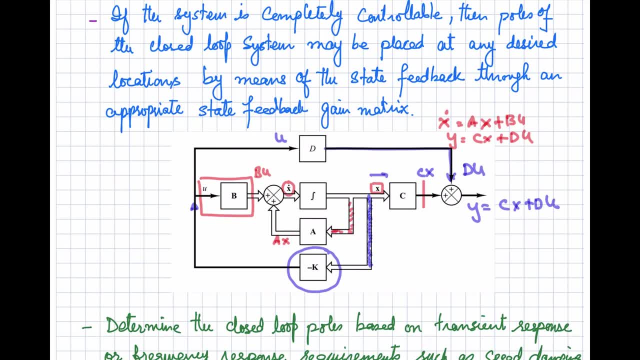 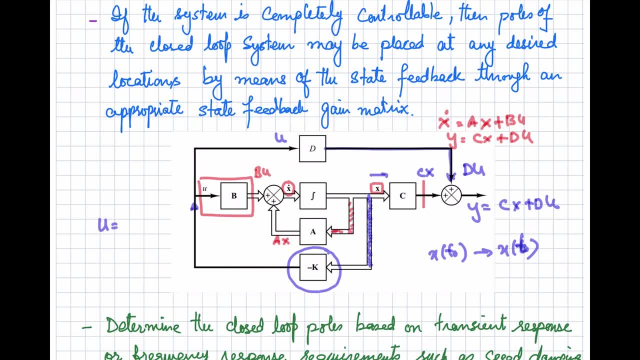 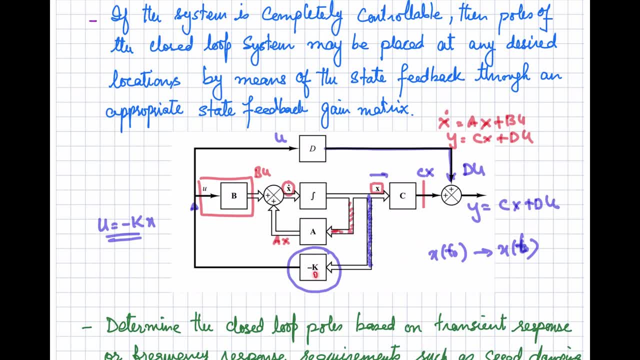 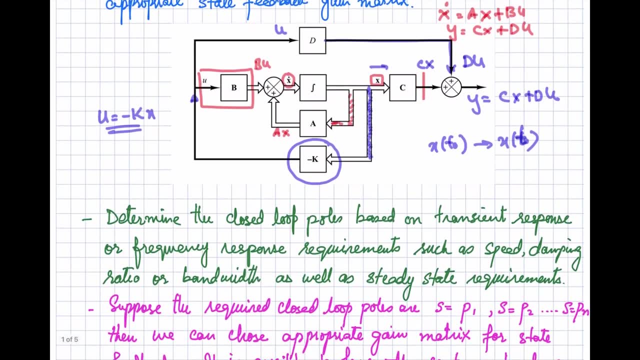 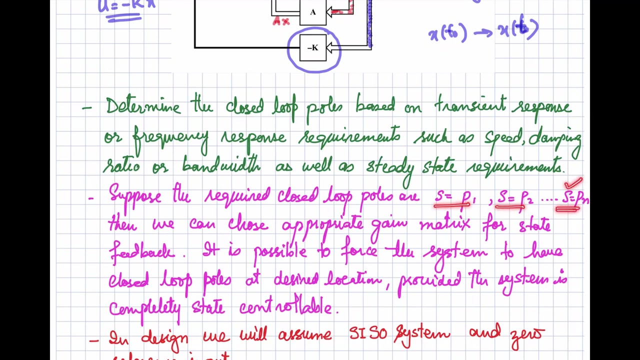 so then it means we can design this controller k. so what is the first step while designing this controller k or this? the let's, let's, let's, let's, let's poles are these ones: s is equal to p1, p2 and up to n number of poles. then we can choose an. 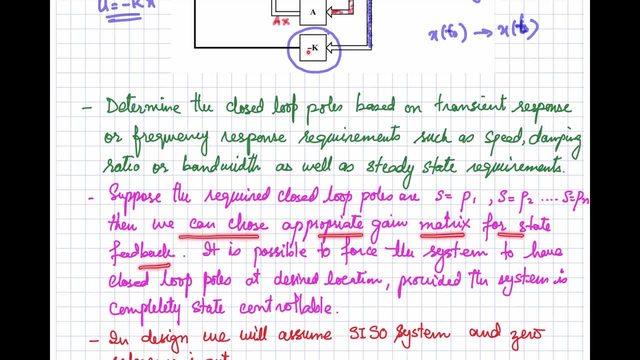 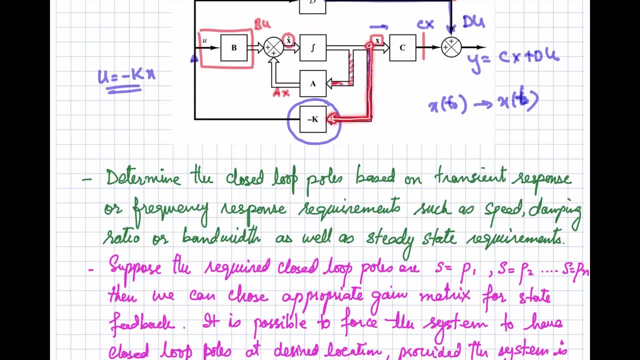 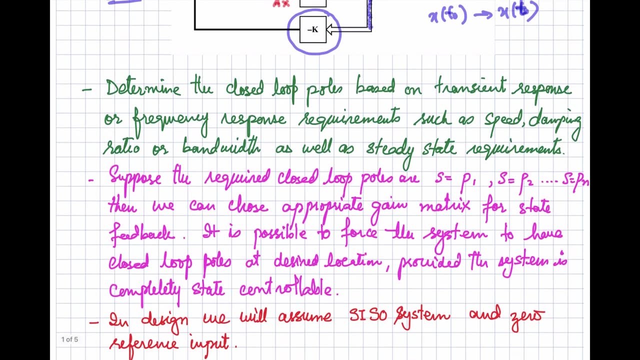 appropriate gain matrix for the state feedback. we are going to call it the state state feedback because we are. you can see, the states are being fed back to construct an input u through this gain k right. so if it is possible to feedback the states through the gain k, then you can adjust. 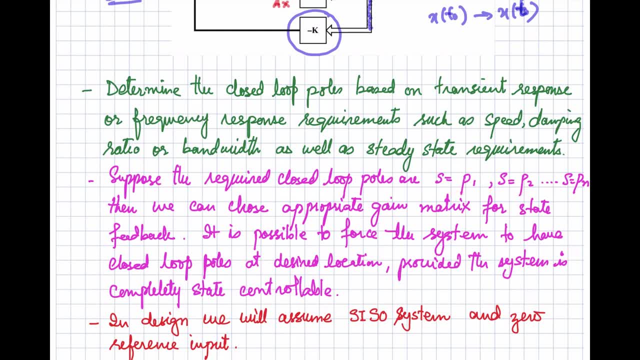 the poles at any desired position. so it is possible to force the system to have the closed loop poles at the desired location, provided your system is completely state controllable. so in order to apply this pole placement method, you will have to check the controllability of 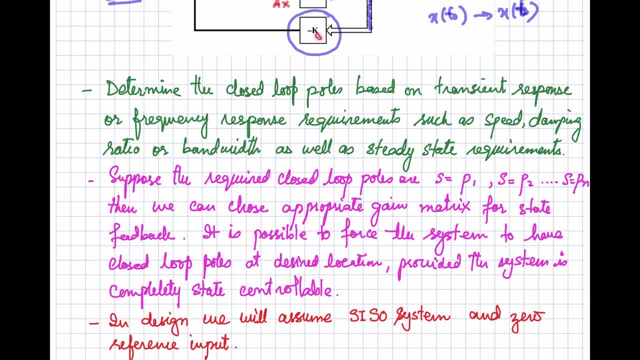 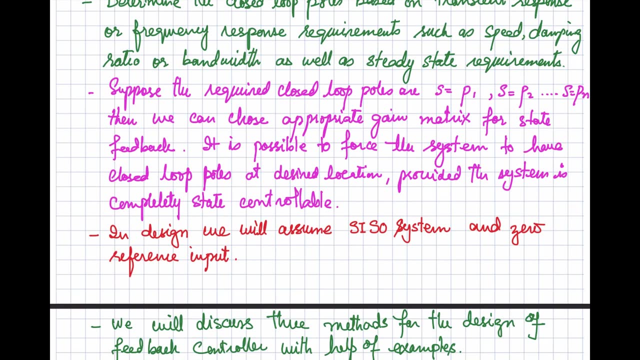 your system. if it is fully controllable, then you can design this block or you can find out the gain of this matrix. in this design we will consider a siso system, single input and single output system, so that all the constants are the scalar ones, and we will assume that that our reference input is. 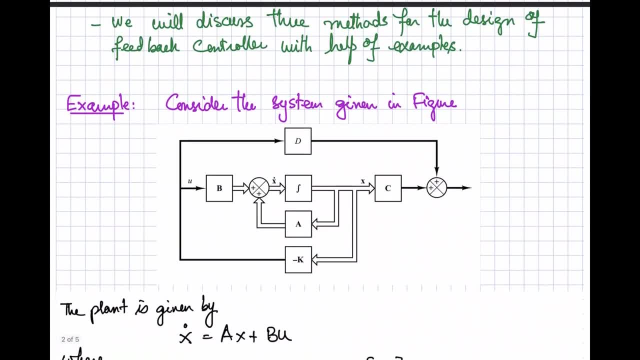 zero. now we will discuss three methods for the design of this feedback controller or to find out the gain of this matrix. so we will consider a siso system, single input and single output system, so that all the constants are the scalar ones, and we will assume that that our reference. 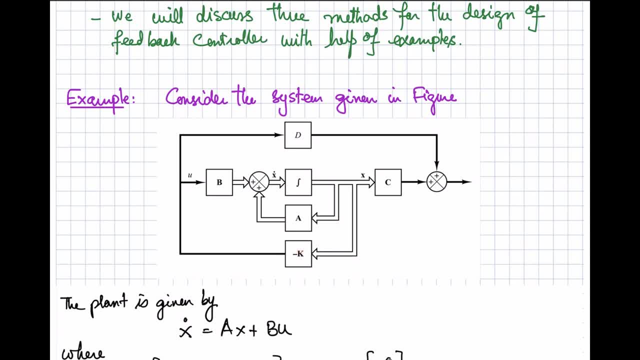 input is zero and in one of these methods we will discuss the appropriate samples for Qualitative Wモl. and the evaluation of the relation between W shall be controlled by a metronome thre, and therefore theあ is not the final shape of the matrix i and. 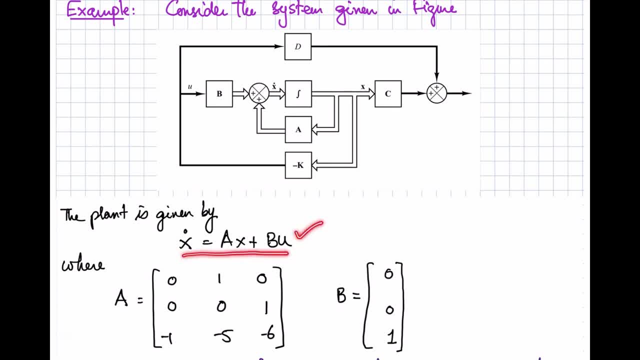 therefore the Del is not the final shape of the matrix i and therefore the Re is not the final shape of the matrix i and therefore the Re is not the final shape of the matrix i and therefore the Re is not the final shape of the matrix i and therefore the Ex matches. Ah, at all these. 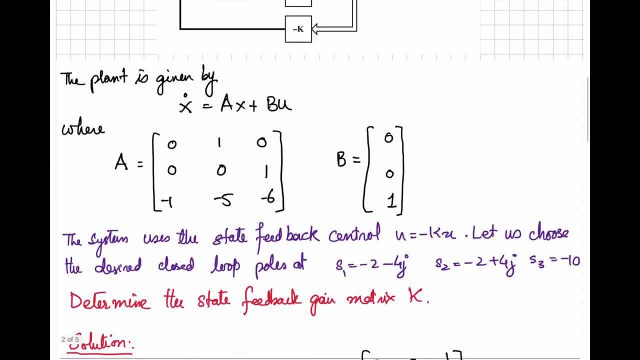 H, s and r s matters. their lugar parameters for the different magnetic fields sound like that of both the R and V même points. so we, the Abergras metres, should be positive. the R is just a function shape, that is Eigen Metronomeerto. So that is a infinite photos. 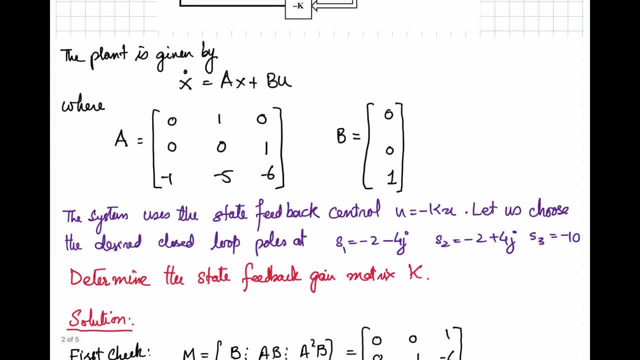 our desired closed loop poles are these ones: first close first pole is at minus 2 minus 4 j. second pole is minus 2 plus 4 j. these are the two conjugate complex pair of the poles right and the third pole is to be placed at. s is equal to minus 10. so these are the desired. 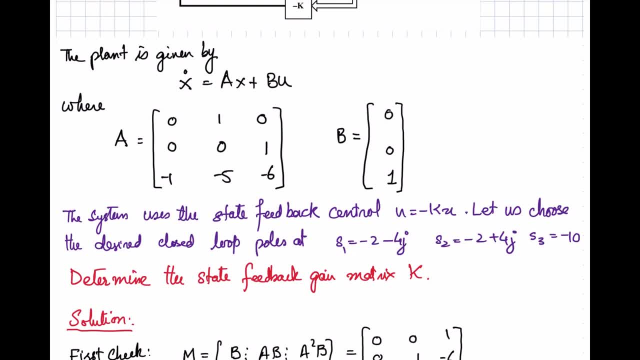 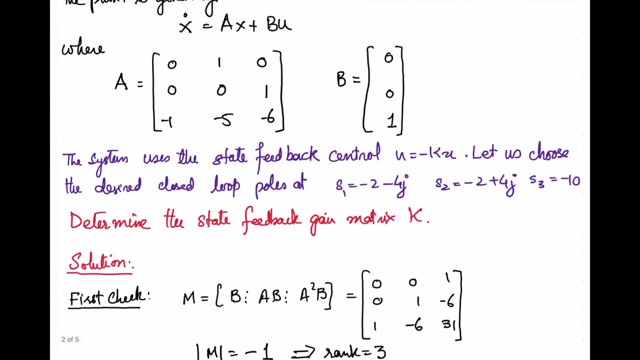 closed loop poles and we are going to use state feedback control. that is, u is equal to minus kx and the requirement is that determine the state feedback matrix k. so i will discuss three methods now with the help of this example. okay, so first method is that that you are going to 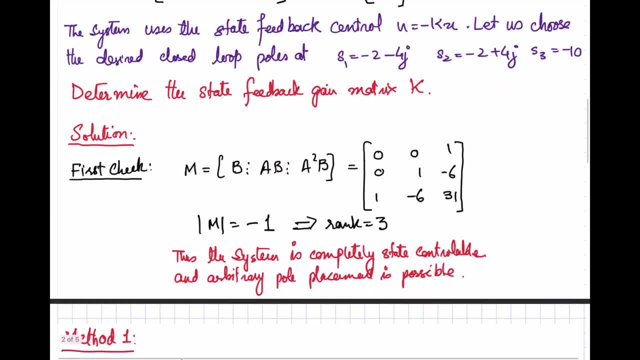 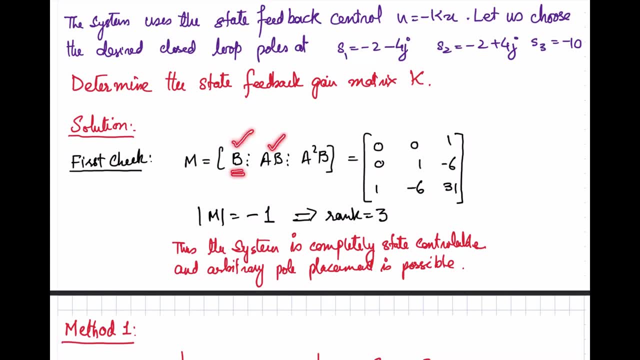 construct a matrix m which consists of input matrix b. the second column is the product of matrix a and b, and the second column is the product of matrix a and b. and the second column is the product of matrix a and b. third column is the product of a square and b and the order of this matrix: the number of columns. 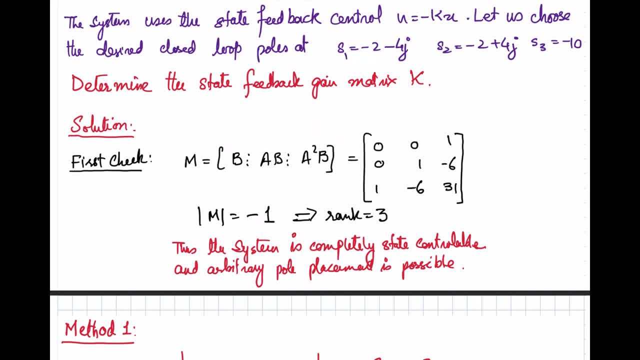 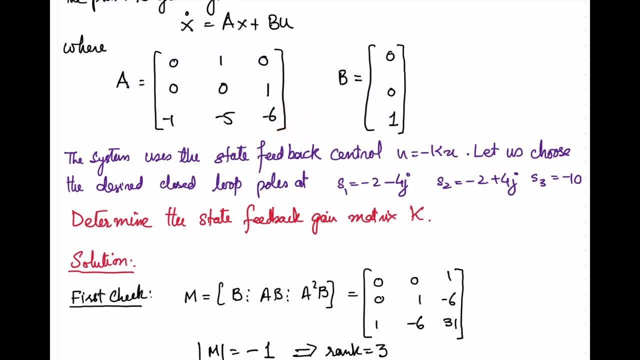 will be equal to n, and what is n? n is basically the order of your matrix a. this is an n cross n and this case is 3 cross 3, so there will be three columns in this matrix. okay, so first of all, you will establish this matrix depending upon the order of your matrix a for 4 cross 4 matrix there. 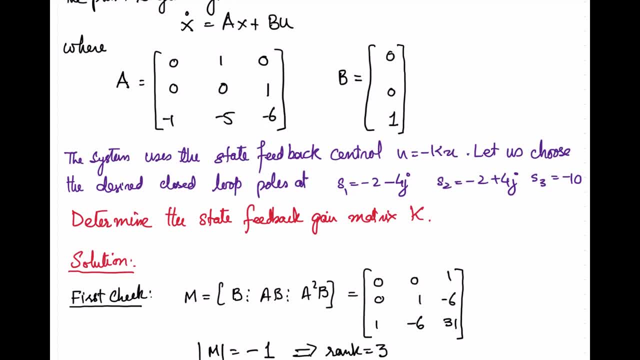 will be another term, a cube into b for higher order matrix. it will be going up to a, n minus 1 into b, where n is the order of this matrix a. so for this particular example, the matrix m is this one, and this must be fully controllable. 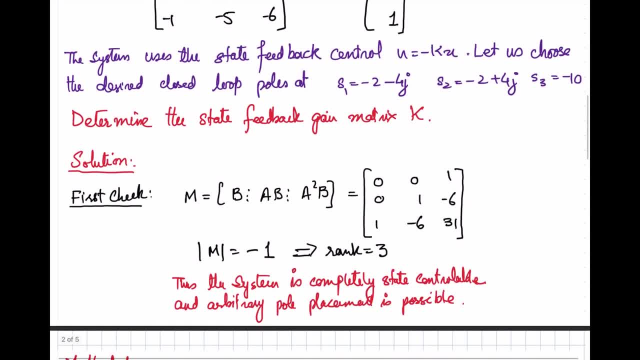 right. so according to the kalman, as we have discussed in the previous videos, this is basically the the matrix a and b and this is the order of the matrix a and b and this is the order of the matrix control ability matrix. so this must not be singular. so if you look at the determinant of 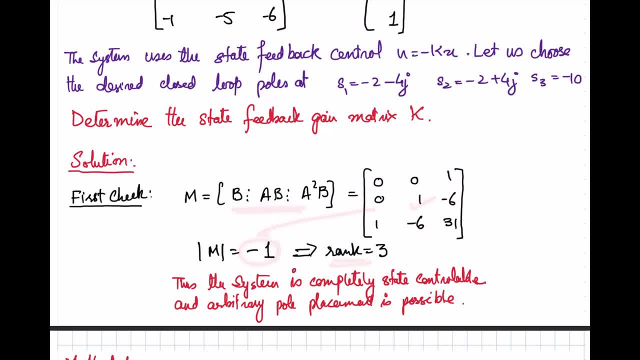 this one determinant is minus 1, so it means the rank of the system is 3, it is fully controllable. and if it is fully controllable, we can place the poles at the desired location by adjusting the gain k in the feedback path right. so now let's discuss the first method, that how we can determine. 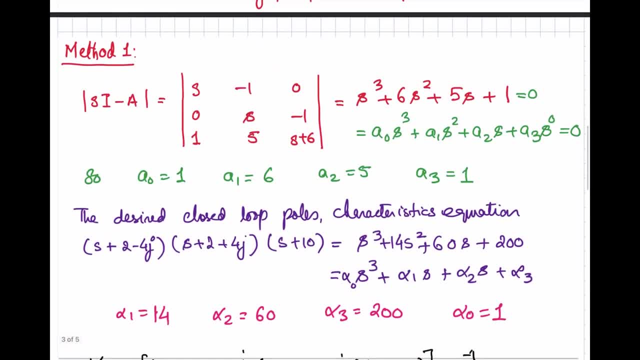 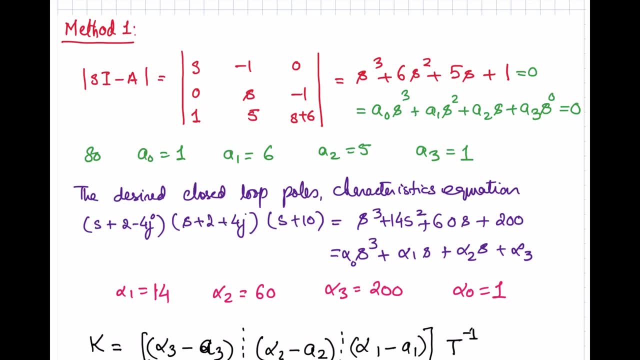 the gain k. the first step was to determine the controllability that we have determined. now we are going to look at it, how we can find out the gain k. so first of all you will have to establish the characteristic equation, that is, s i minus a, or this equation in s domain. 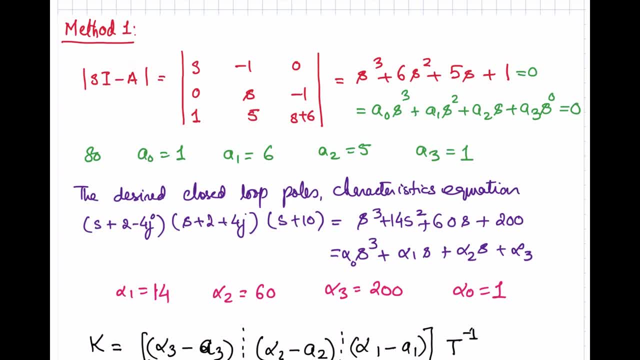 so you know the matrix a, so i is the identity matrix, so you can set up this determinant and from here you are going to find out the characteristic equation and you are going to set it equal to zero. so this term is being compared with the generic third order equation. let's suppose a naught sq plus. 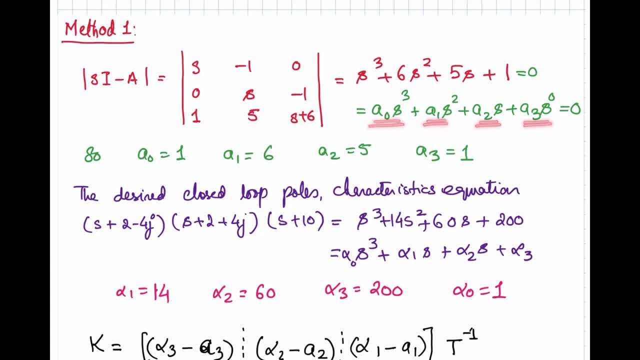 a 1 sq plus a 2 s plus a 3 s, naught all of these, and this is s power 0 s, power 1 s, power 2 s, power 3. this is our variable and these are the constants. so if we compare this equation with this one, i can: 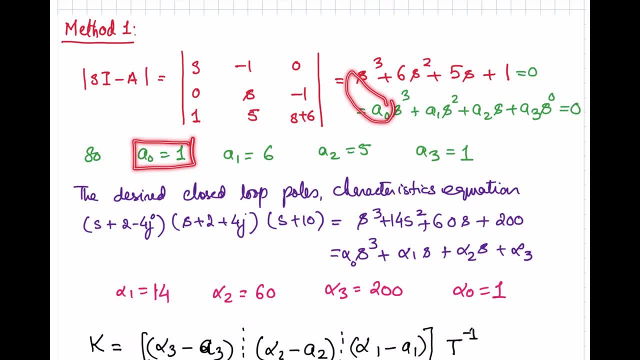 say, a naught is equal to 1. by this comparison, a 1 is equal to 6, a 2 is equal to 5 and a 3 is equal to 1. so we have specified these values of a naught: a 1, a 2 and a 3. now we are going to develop the 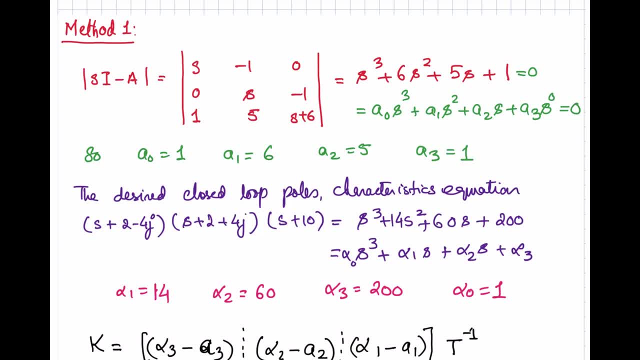 characteristic equation with the help of the uh, with the help of the given closed loop poles. so these are the closed loop poles. if you multiply these ones, so you will get the characteristic equation. so if we multiply all of these, we are going to get this equation. and 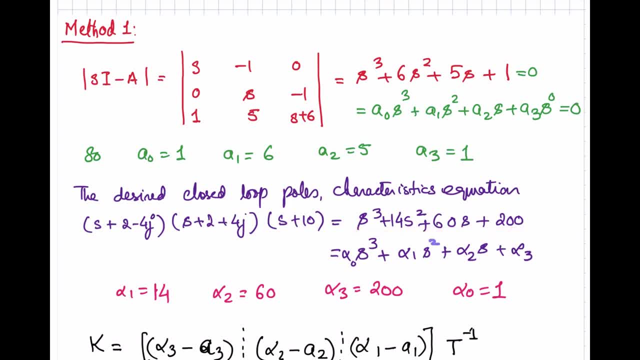 again, if you look at the standard equation, let's suppose alpha 0 s cube, alpha 1 s squared, alpha 2 s and alpha 3 s power 0, so you can find out the values of the alpha, alpha 1, alpha 2, alpha 3 and alpha. 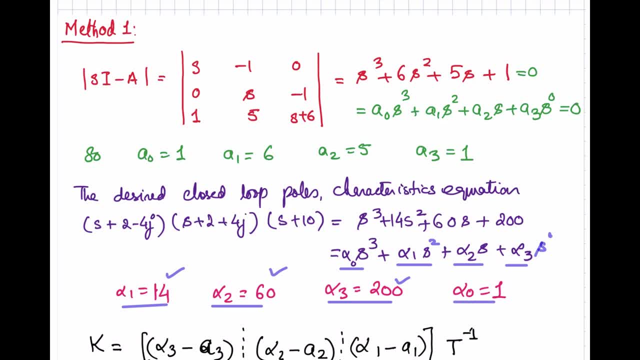 naught right. so we have obtained it by comparing: alpha naught is equal to 1, reason: alpha 1 is equal to 14, alpha 2 is equal to 60 and alpha 3 is equal to 200. so once you have obtained these ones, these are the coefficients of the actual characteristic. 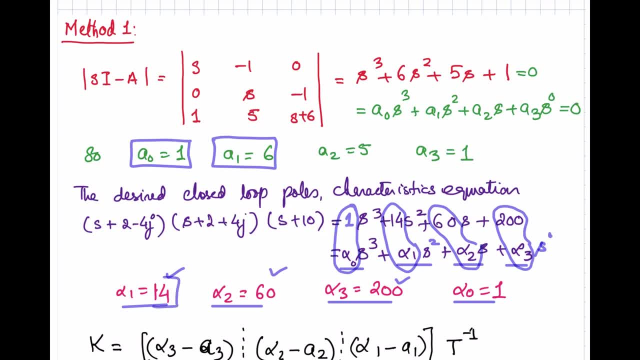 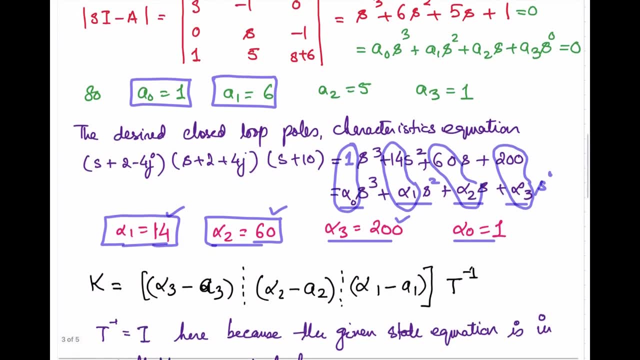 equation and these are the coefficients in the desired characteristic equation. so the first method is that that you can determine the gain k with the help of this equation. that is, the k is equal to alpha 3 minus a3. this is the desired coefficient, this is the actual. 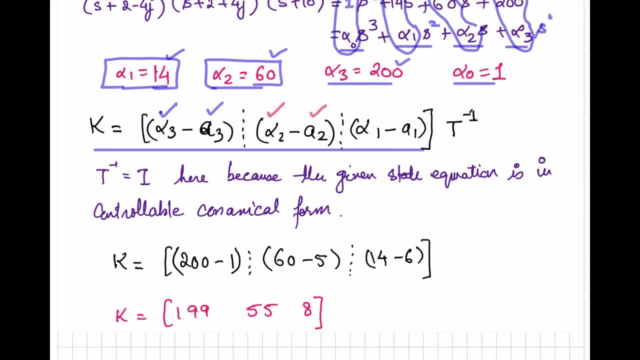 coefficient. similarly, this is desired coefficient, this is the actual coefficient, desired coefficient, and the actual coefficient into t minus 1 and t inverse. what is this? t inverse- t inverse, basically is the transform method and this is the transform method and this is the transform method, and this. 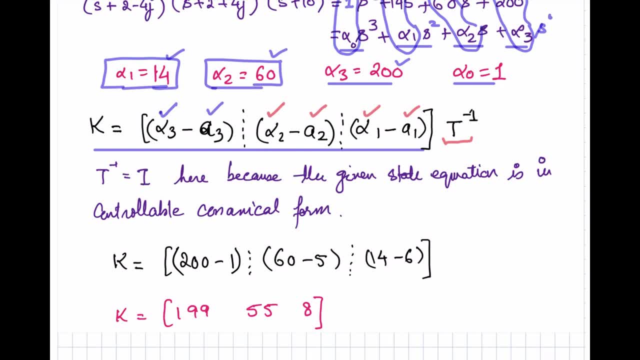 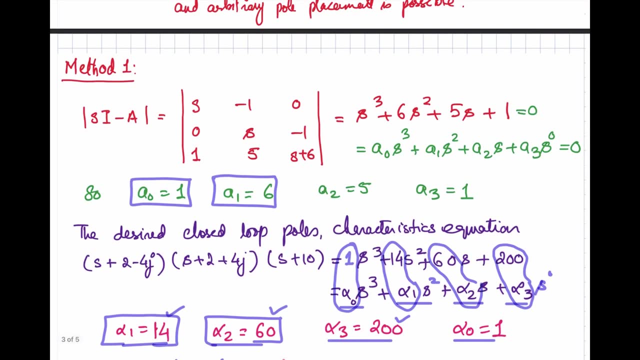 transformation. if your system is not in the canonical form, then through that transformation, first of all you will have to bring your system, matrix a, into the canonical form. over here it is given as it is given to us in the canonical form. if you look at that one, that matrix a, it is in 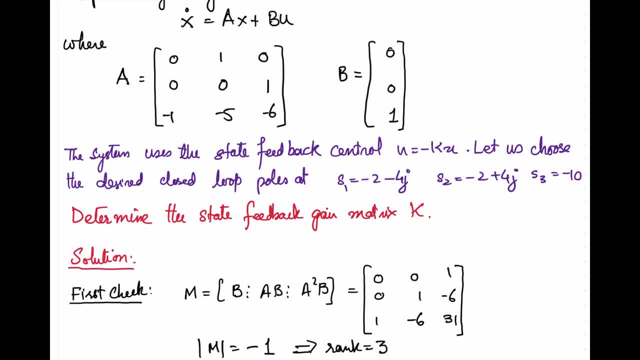 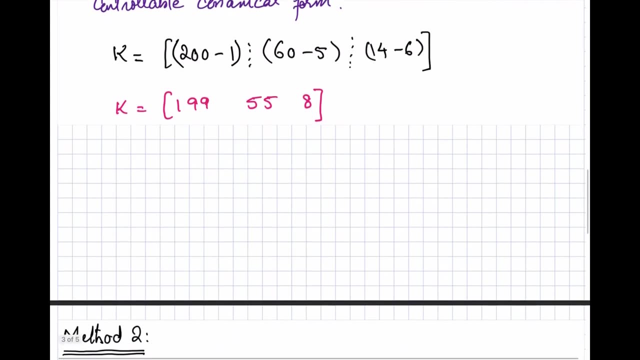 the canonical form, right, so that's why this, the matrix t inverse, will be equal to identity matrix, because it is already in the canonical form. otherwise you will have to bring it in the canonical form. okay, so once you determine these values, the coefficients of the desired and the 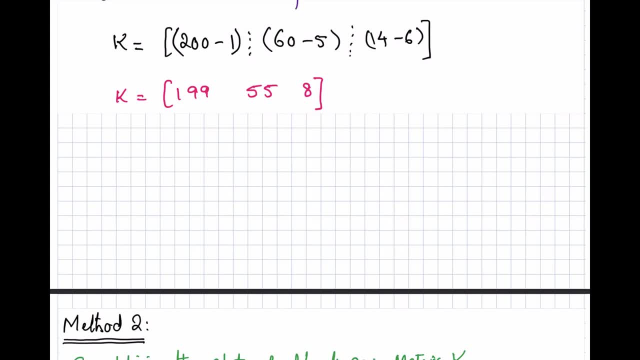 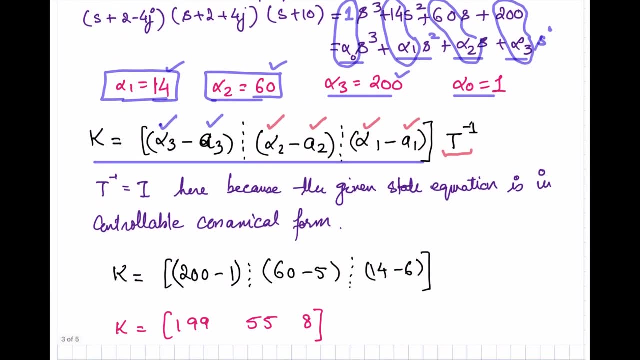 actual characteristic equation. so then, with the help of this equation k, you can determine the gain k. so in this case, this t inverse is identity matrix, because we have already, in the controllable form, in the canonical form, so directly by using the values, the desired value and the actual value. 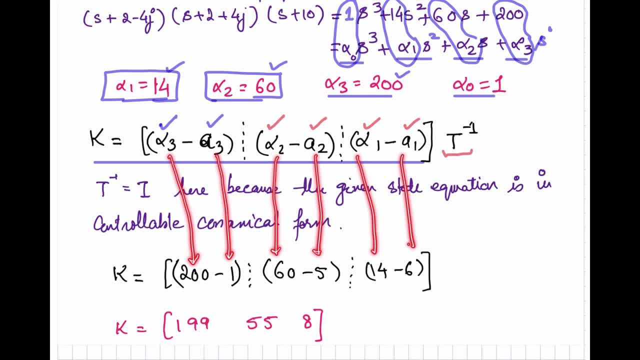 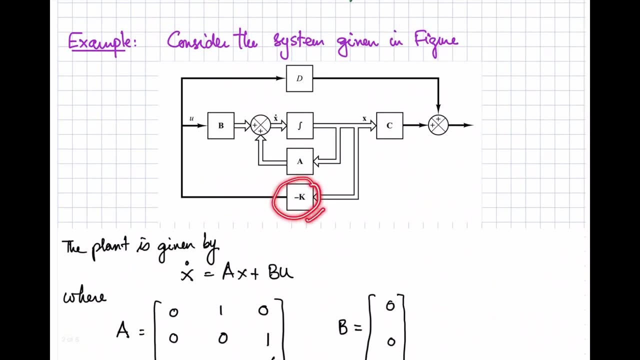 desired value and the actual value and so on, so you can obtain this matrix k, that is one 99,55,8. this will be the gain of your feedback path. this one, this k will be adjusted equal to this one, so that you are going to have the required input that will adjust the closed loop. 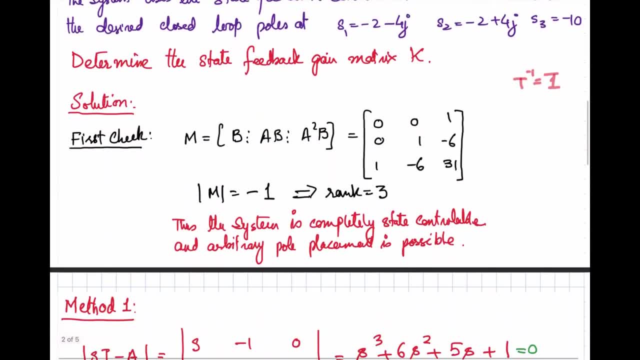 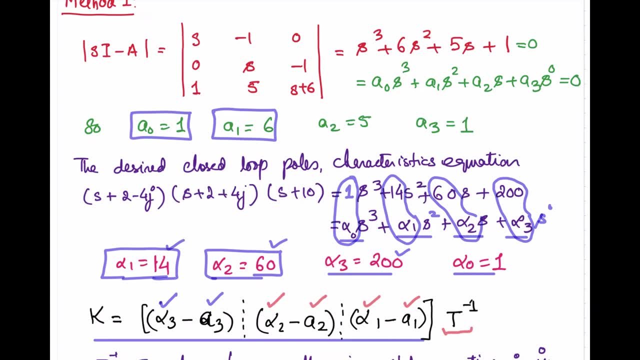 poles at the desired position. so this is the first method. what is that? if i summarize, set up OK. so we have to have the characteristic equation of the given system. right k means 1 for each one of them, which is equal to k plus mod k for each of the keys, and that will be appropriate for every distribution of the game. 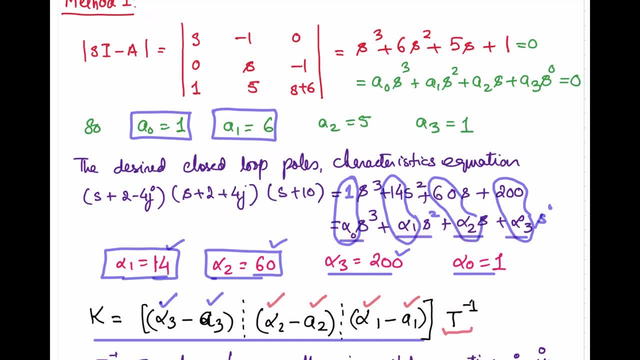 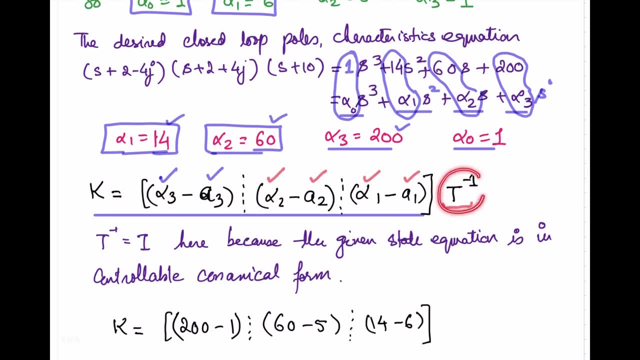 then the desired system find out the difference of the coefficients. and those differences will be the gains if your matrix is directly in the canonical form. otherwise you will have to multiply it with the transformation matrix to bring it into the controllable form. sorry, canonical form. okay, now let's look at the second method. 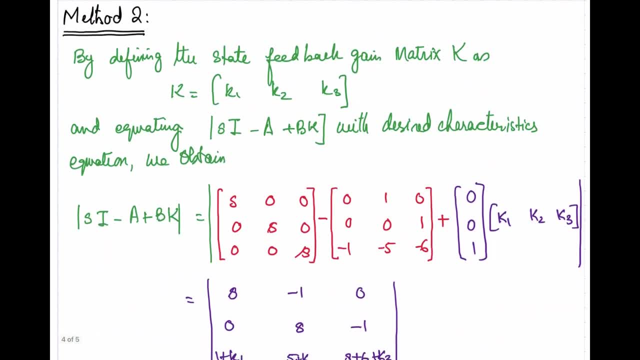 so in this we are going to define the state state feedback matrix k like this: k is equal to k1, k2 and k3 and in this we will use this equation, s into i minus a plus bk, and we will compare this equation with the desired characteristic equation. 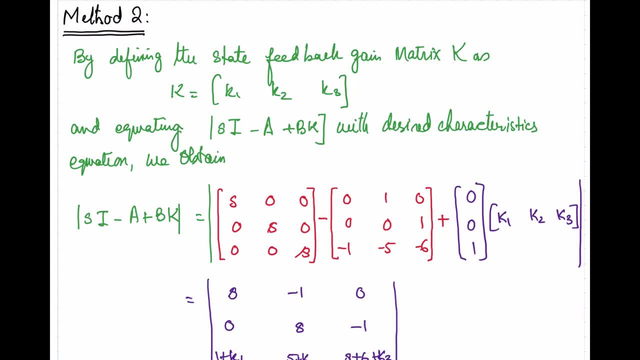 to look at the required gain k. so first of all, we are going to set up this equation: s i minus a plus bk. so this is the matrix s i, this is matrix a, this is matrix b and this is matrix k. so all of these are the matrices. what is this k matrix that we assumed over here again? 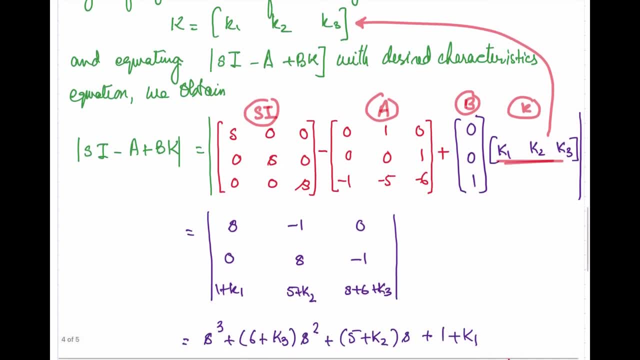 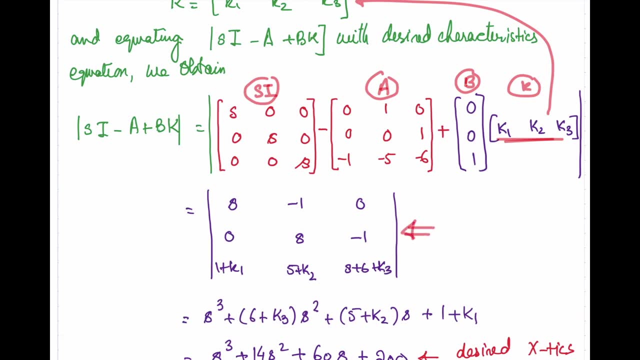 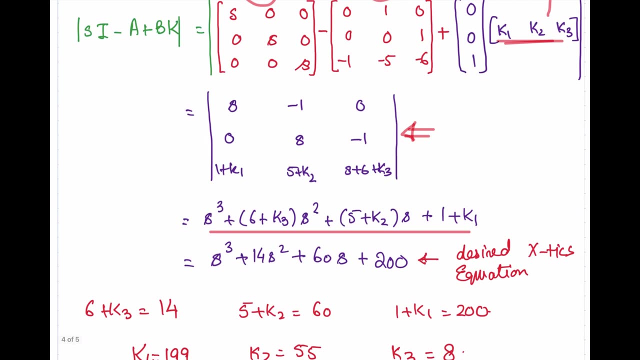 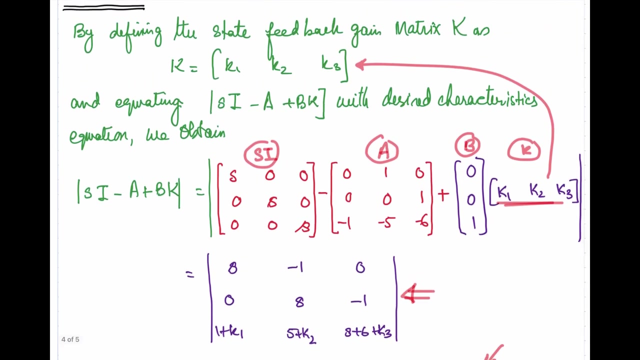 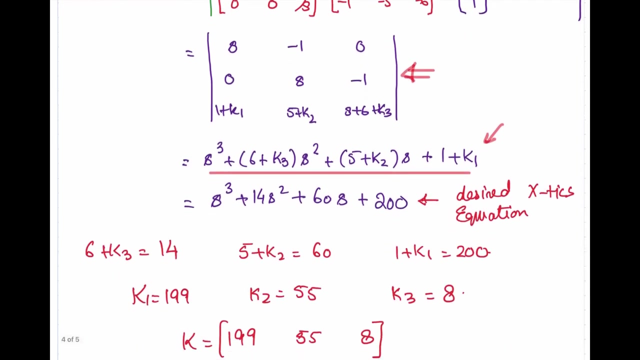 matrix k. so now, with the help of this, we are going to set up an equation, and that is this one. so, evaluating this determinant, we can write this equation right, and this is the equation that we obtained by setting up this equation, this characteristic equation, and we have seen the desired characteristic equation before that was. 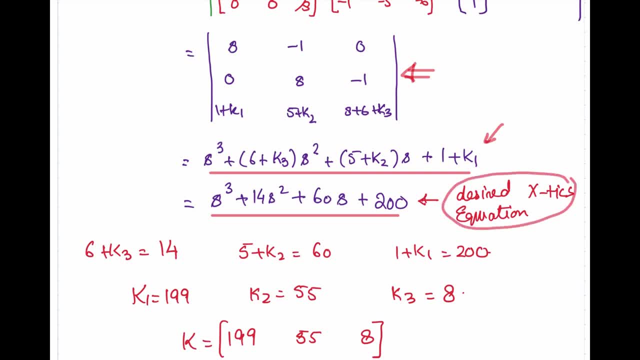 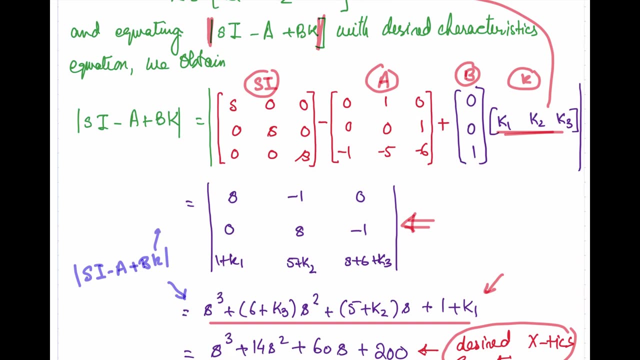 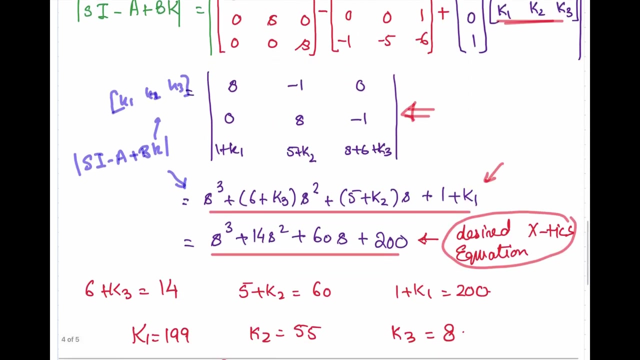 this one. this is the desired characteristic equation, and this is the characteristic equation that we have obtained by setting up this one right, where this k is the matrix consisting of k1, k2 and k3. okay, so now again, we are going to compare the coefficients of the desired and the actual. 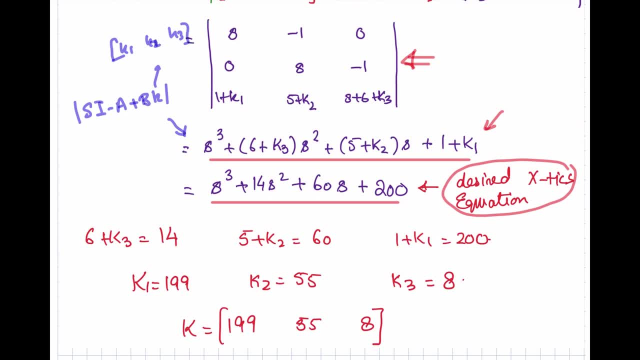 characteristic equation. this one is the desired in the desired. with s3 we have one. in the actual, we have the one no difference in. in the term s-square, the desired value is 14 and that is to be set equal to 6 plus k3. so 6 plus k3 is equal to 14. so we have one equation. this is the deserved one, okay, and we are to calculate the an. estão o deco mujer. esta novato, tudo angel é de wishar que ele se contrata. use a categorizado com tek höher a số maior. 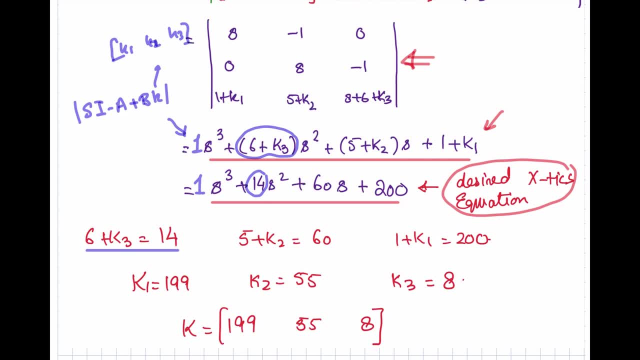 so that is to be set equal to 6 plus k 3. so 6 plus k 3 is equal to 14. so we are left with an equation. дальшеko是 figured的. from here we can find out: k3. k3 will be equal to 8. now, by comparing these, 5 plus k2 should be. 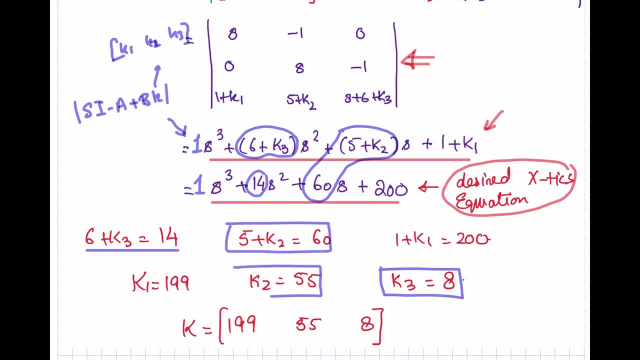 equal to 60. so from here we can find out k2. k2 will be equal to 55, and then this 1 plus k should be equal to 200. so from this equation you can find out k1 that is equal to 199. so again you can see. 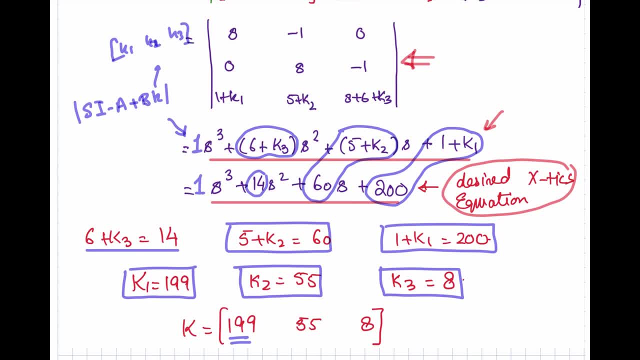 we are going to get the same gain matrix that we obtained in the first method. it consists of three elements: k1, k2 and k3. k1 is 199, k2 is 55 and k3 is 8. it is exactly same what we obtained. 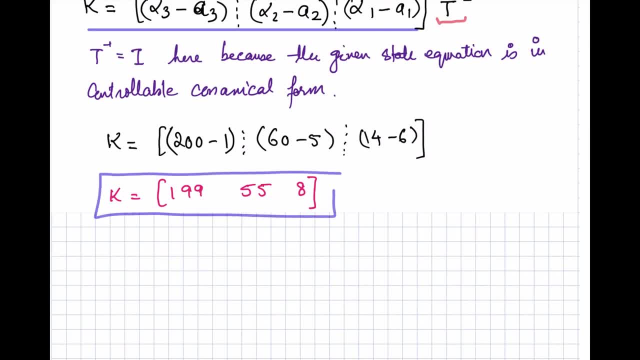 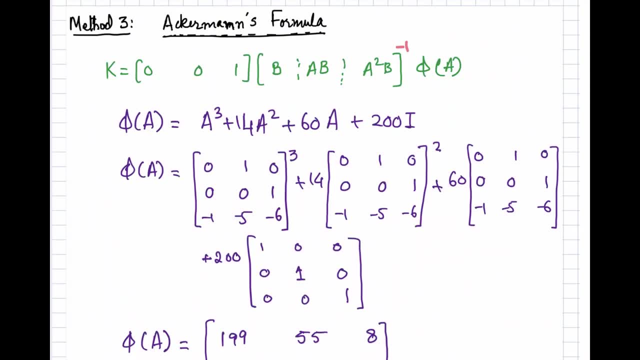 over here in the first method, right, so you can use either first or the second method to determine the gain k. so now let's look at the method 3. in this method we basically use the eckermann's formula to determine the gain k. so the gain k is given by this equation. 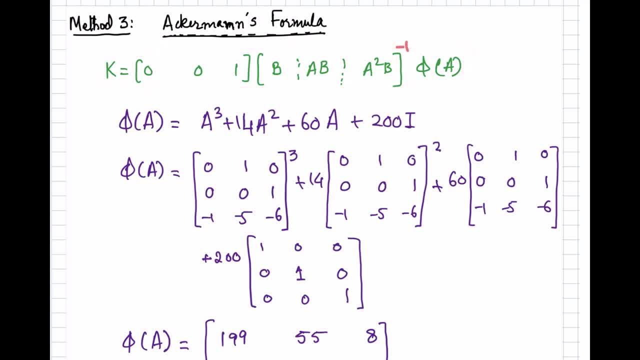 the first part of this equation is this matrix: it consists of all zeros except the last 20. that is equal to 1, and this is your controllability matrix. now let's look at the method 3. in this method, we basically use the eckerman's formula to determine. 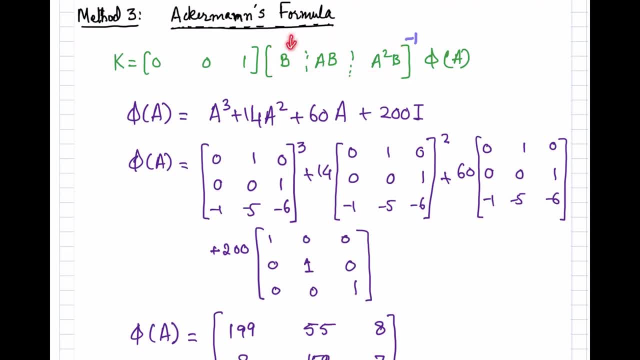 the gain k. so the first column consists of b. the second- sorry first- column consists of b. the second column is the product of a- b. the third column is a square b. it depends upon the order. over here we have the three cross, three matrix. so for that's why we have the maximum power, 2, because this is. 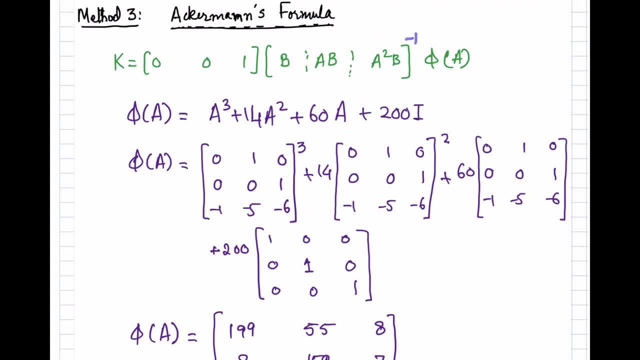 equal to n minus 1 in the controllability matrix. so we are going to take the inverse of the controllability matrix over here, right? so why we are going to take the controllability matrix? because we have seen earlier there that pole placement method is only possible. 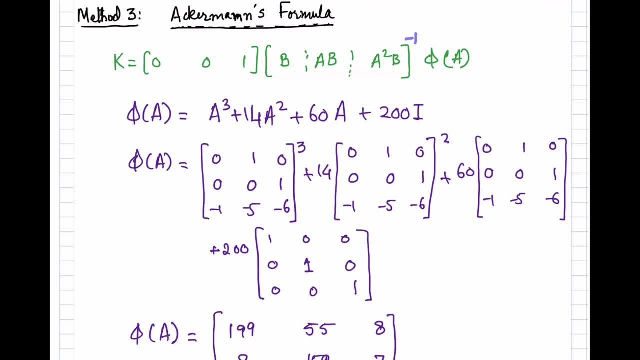 if your system is completely controllable, then you can define an unconstrained input which will give you the transition from the state x t naught to some other state x t in a finite amount of time. and what is this? phi a, this is the finite amount of time of time that we have to have in order to determine the gain k. so this is the finite amount of time that we have to have in order to determine the gain k. 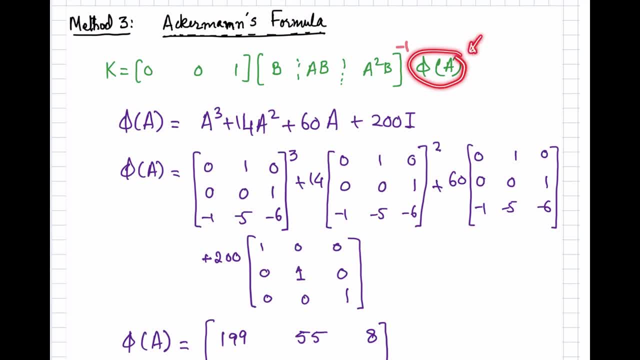 This is the desired characteristic equation in terms of A. We have already seen that. that what we require, what equation is required or desired as the characteristic equation? If I write that one over here, so that was equal to S cube plus 14 S square plus 60 S plus 200.. We have seen it above. 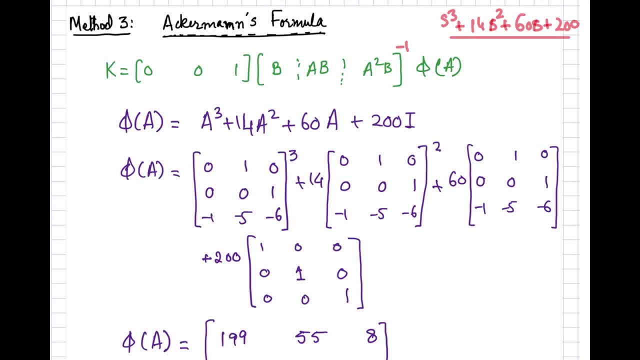 this is the desired characteristic equation, So we are going to write it in terms of A, the matrix A. So here you can see, this S cube will give you A cube. 14 S square means 14 S square. 14 S square is equal to 14 S square, So we are going to write it in terms of A. 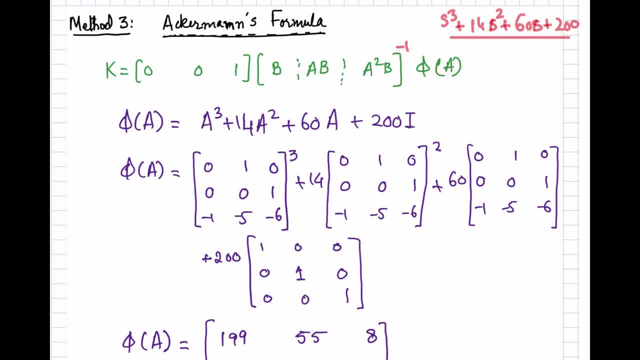 60 A and the 200 as it is to be written in the matrix form. So we will have to use the identity matrix over here, Right. So now let's calculate first of all this equation. Let's place the value of the A. We know the A from the given information The system is given to us. This is matrix A. 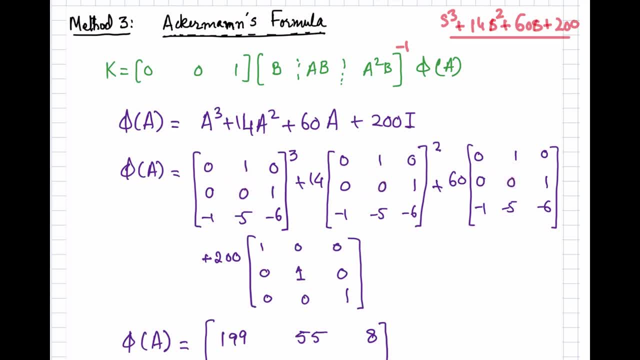 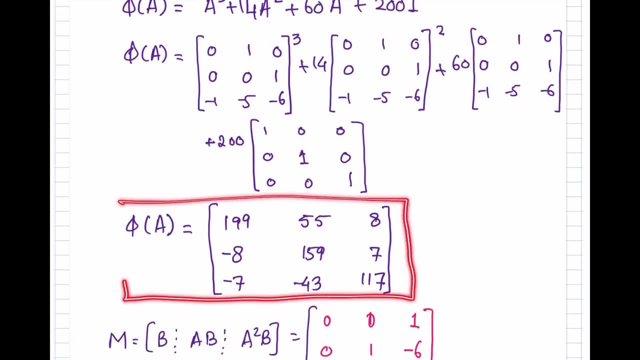 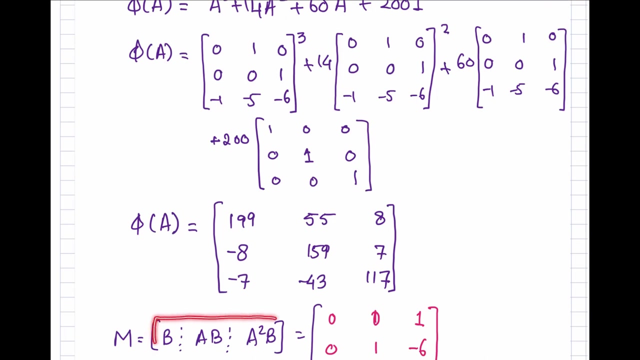 All of these ones. So, after simplifying, we are going to get this matrix. This is phi A matrix, The required characteristic equation in terms of A. So we have obtained this matrix. Now let's calculate the controllability matrix. So controllability matrix is given by this matrix, That is B. 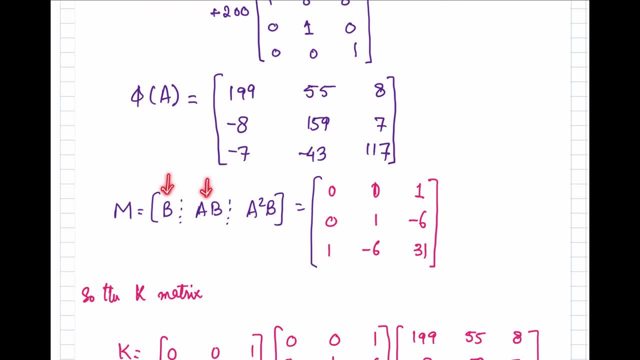 First column is b, second is a b and the third one is a square b. so this is b, the product of a and b. is this one 0, 1 and minus 6, and the product of a square with b. is this column right? so this is the controllability. 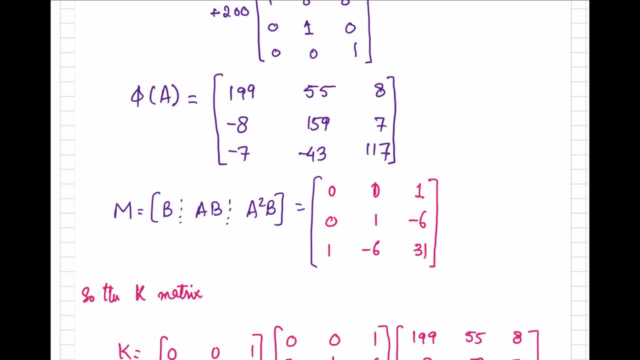 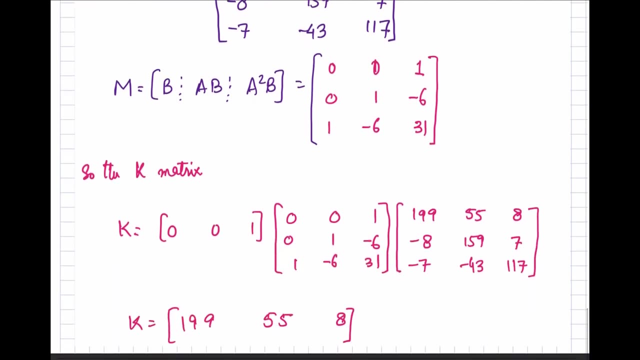 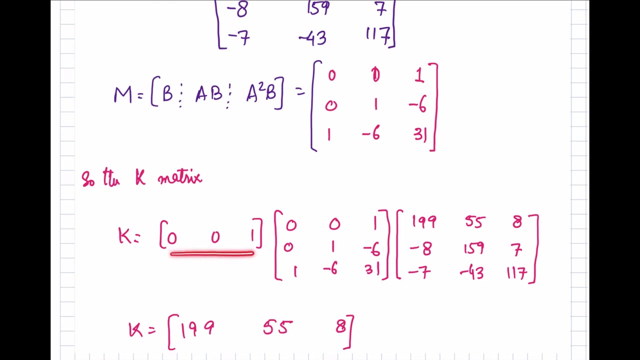 matrix. now we know the phi a, which is the characteristic equation in terms of a, and we have the controllability matrix. now we can find out the gain matrix k just by multiplying 0, 0, 1 inverse of the controllability matrix and phi a.